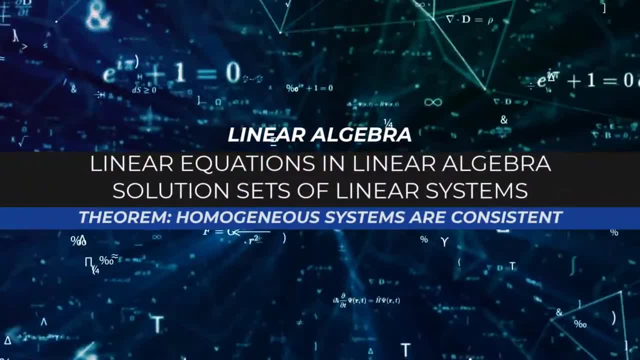 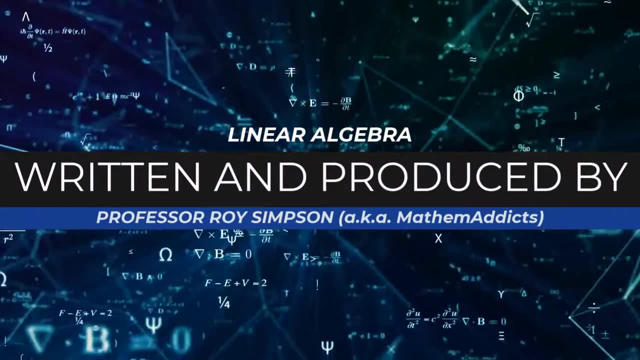 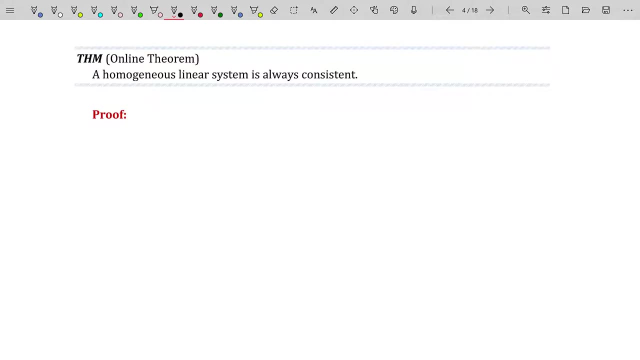 Hello, my name is Roy Simpson, Professor of Mathematics at Cosumnes River College in Sacramento, California. In this video, which is dedicated to Linear Algebra students, we're going to start talking about homogeneous linear systems, specifically the fact that they're always 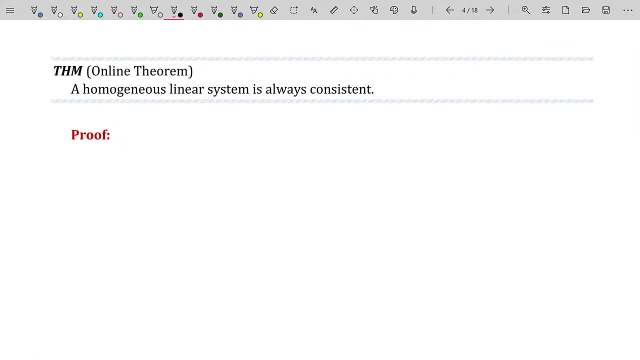 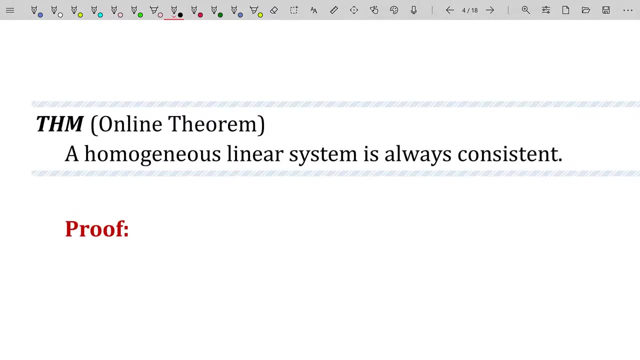 consistent. So this is just focused on one simple theorem here, very fast, we're also going to prove it. but the theorem is just that A homogeneous linear system is always consistent. Remember, a system of linear equations is said to be homogeneous if it can be written. 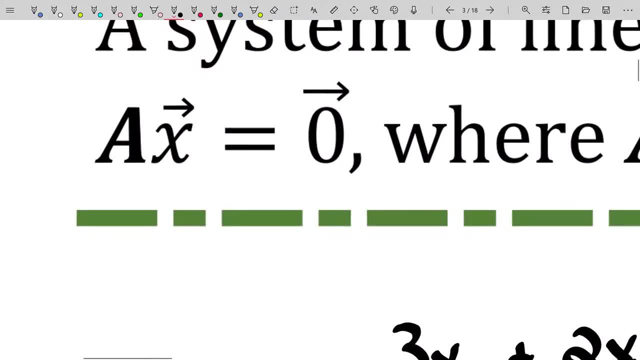 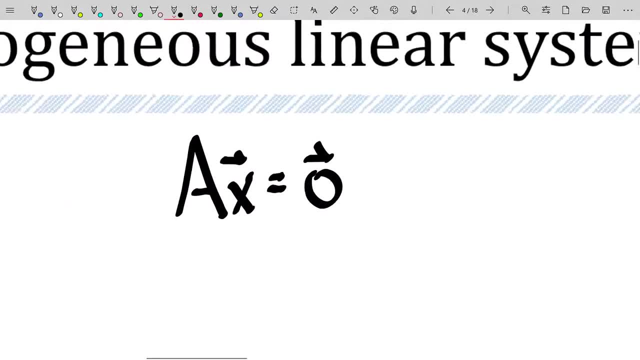 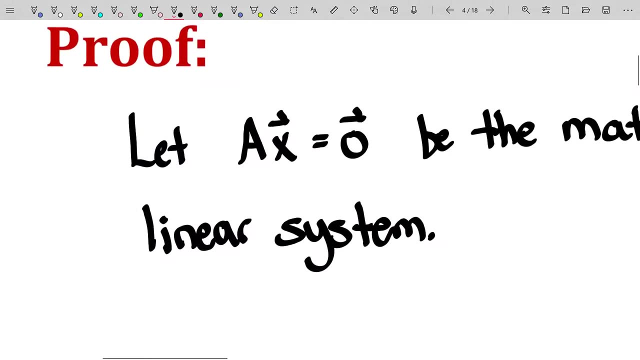 in the form Ax equals zero when you write it as a matrix equation. So again, the claim is that the system associated with this matrix equation is always consistent. We'll start our proof with the statement that we're going to let Ax equals zero be the matrix. 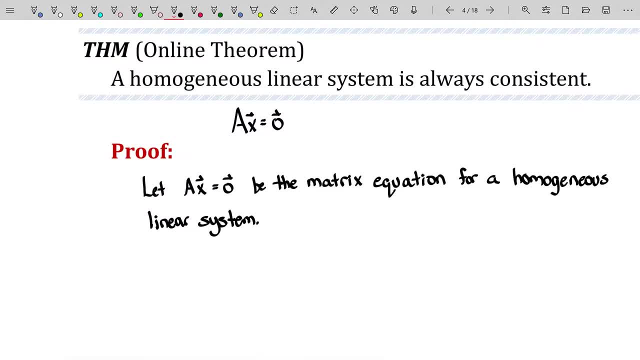 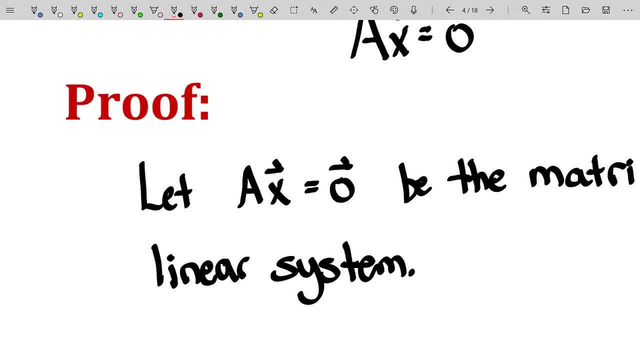 equation for a homogeneous linear system. It's kind of a given actually if you write Ax equals zero, like that, the matrix being A and we have a solution, vector x and a right-hand side vector zero, And what we want to showcase is that has a solution and this is going. 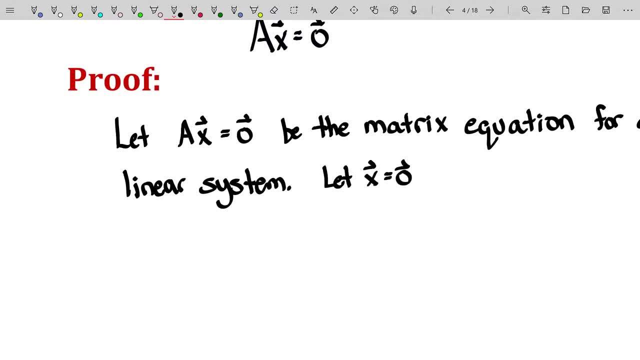 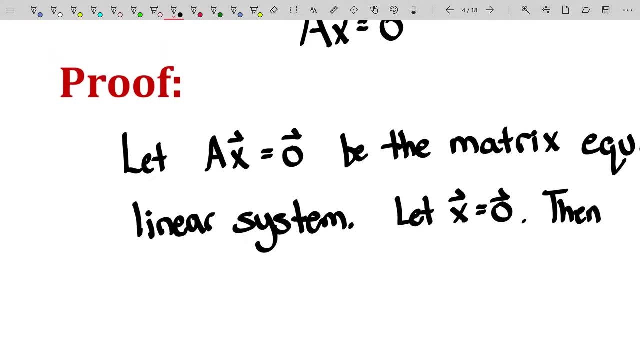 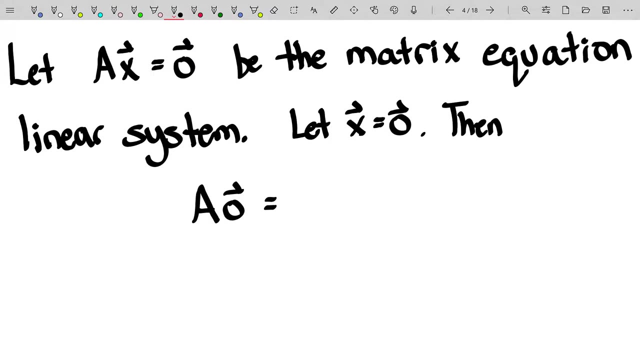 to be very fast, We're just going to let x equals zero where the size of the zero vector matrix multiplication makes sense. If that's the case, then the matrix A times the vector zero will equal a linear combination of the columns of A, where the weights of those column 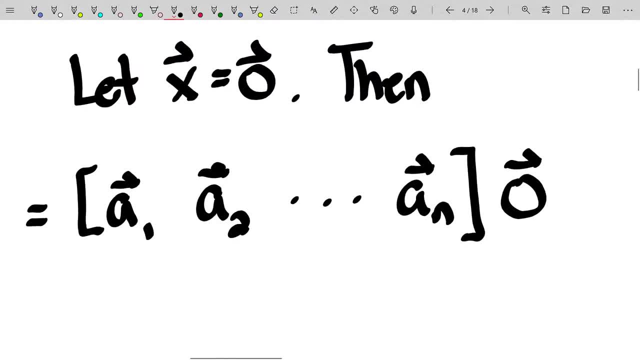 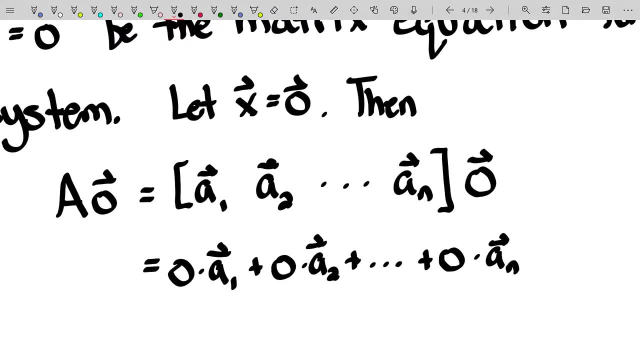 vectors are set by the entries in the zero vector, which, by the way, are all zero. Obviously, we're assuming that, again, zero is in Rn, because there has to be n entries in zero for it to match the number of columns in A. 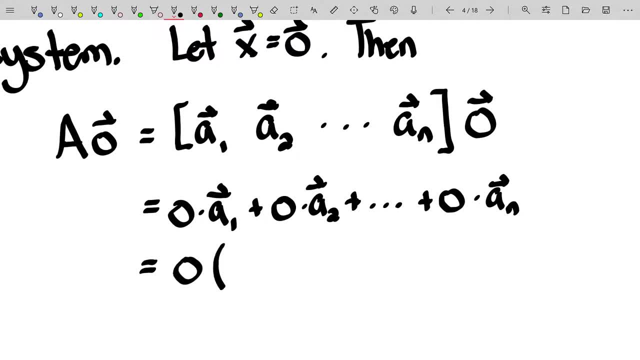 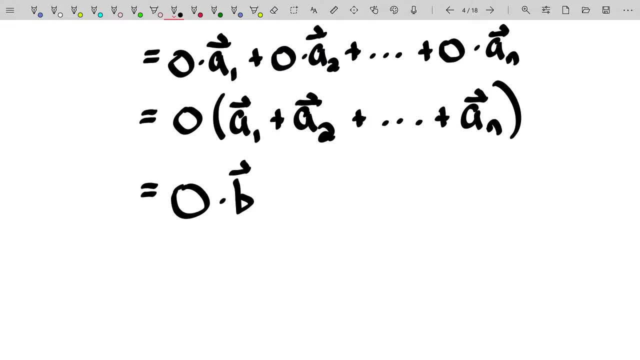 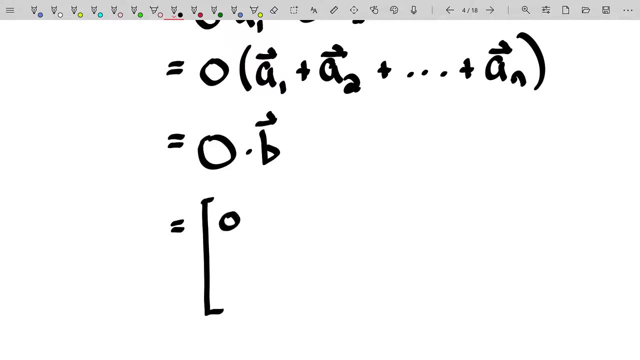 You could factor a zero out of all of those. That summation of the column vectors of A becomes some other vector. We'll call it B for now and then zero the scalar times. the vector B means that you'll end up with a vector zero times B sub one zero times.